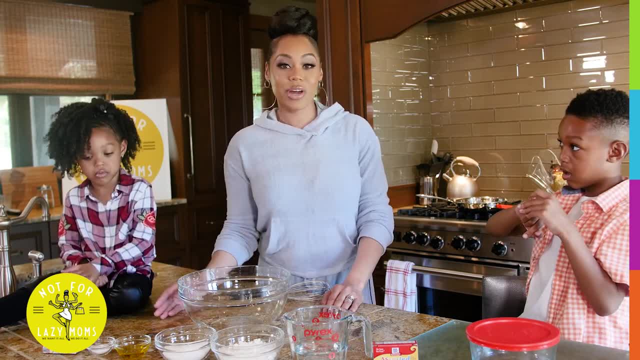 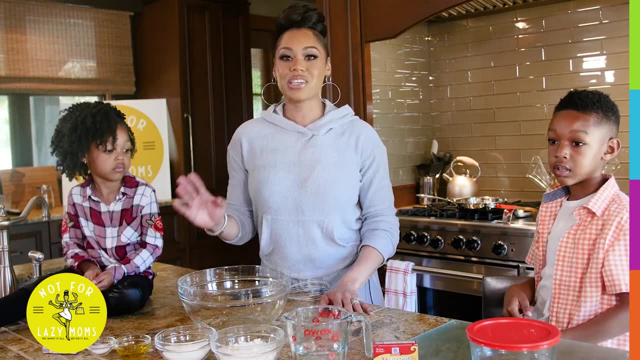 what ingredients were in the Play-Doh that you buy from the store. So I wanted to make sure I had ingredients that were edible, just in case they were to put some in their mouth. So I don't encourage them to eat it, but it just helps to know that if they were to take a little taste. 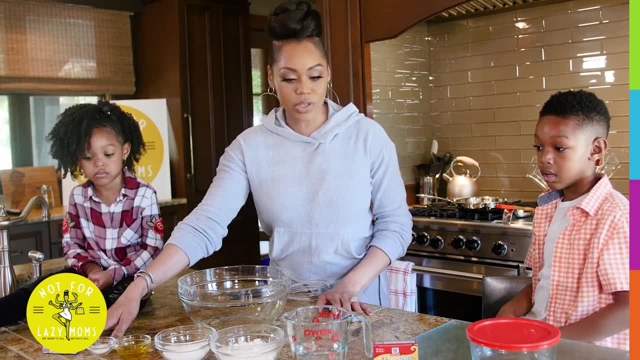 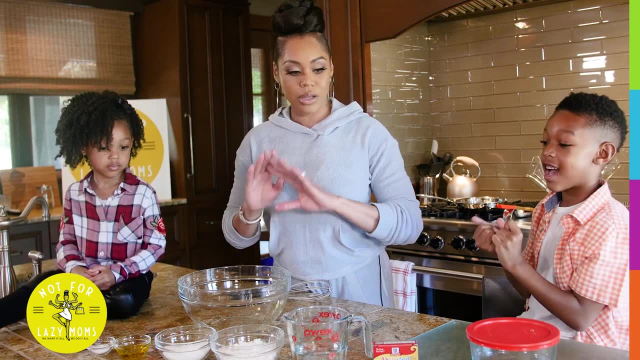 it's not going to kill them. And then we also have the food coloring. So what color are we going to make today? You want to make purple? Can we do that? Okay, so we'll make purple, but we'll use the food coloring, Yeah. ingredients: 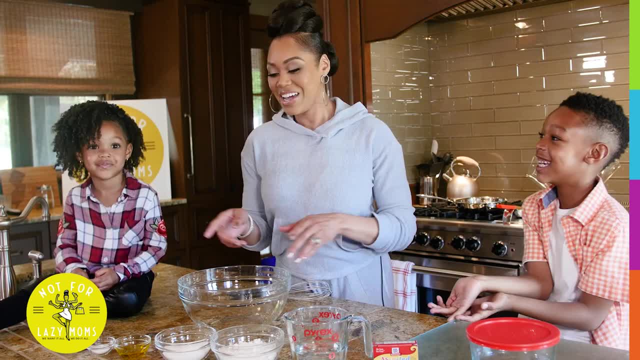 Ingredients, ingredients- All right, ingredients. you silly behind? Okay, all right. so now we need to put what in the pot. You want to put the cream of tartar in here? Yeah, cream of tartar, All right. 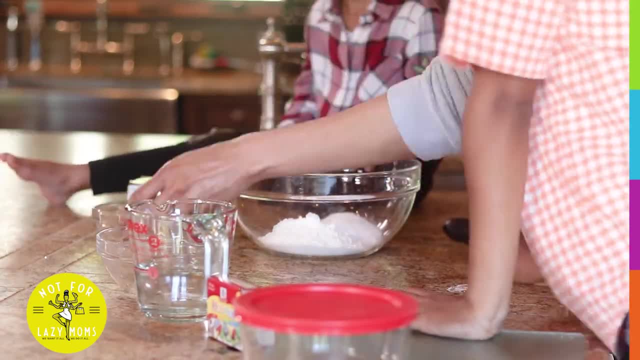 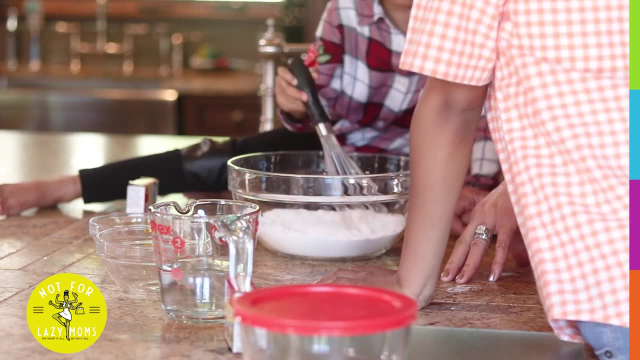 you put the flour in. Go ahead and let's put all of that inside the bowl. Don't dump it too high so that it doesn't get all over the place. You have to put all of it And the flour. you need to, yeah, dump the whole thing. The best way to keep kids occupied is to let them help. So these 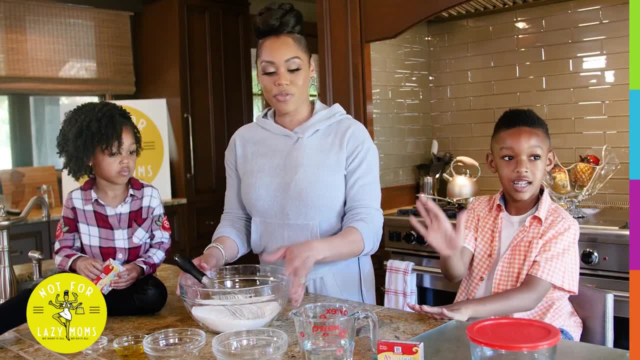 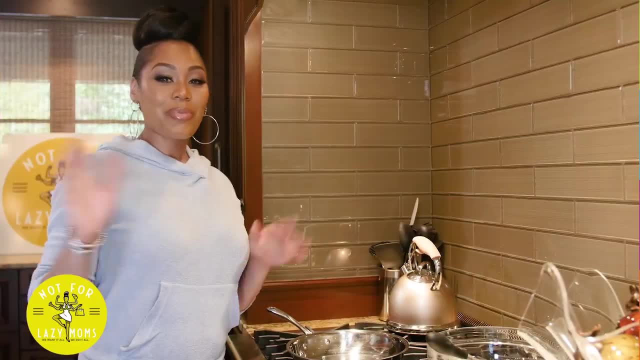 are my little helpers, right. So now we're going to take the ingredients to the stove and then I'll add in the water and the olive oil And the food coloring right away. So now I'm going to let the kids have a break and I'm going to 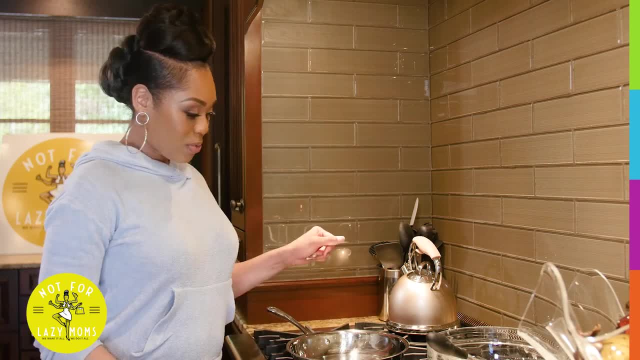 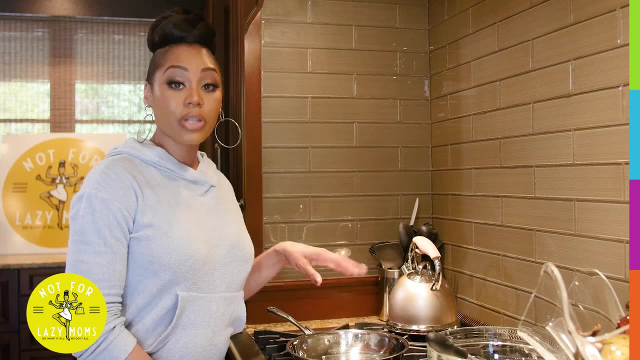 actually put everything on the stove, keep them away from the fire and we'll mix all the ingredients and see how it turns out. So the first thing you want to do is turn your fire on very low heat. It cooks really fast, so you'd be surprised. You don't want the pan too hot. First thing you'll 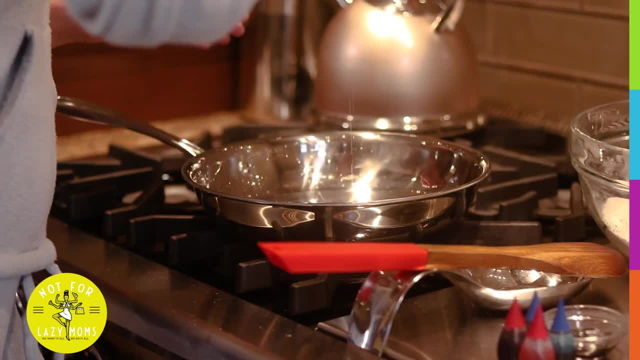 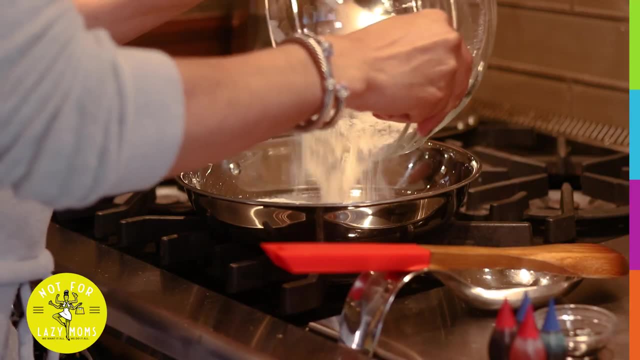 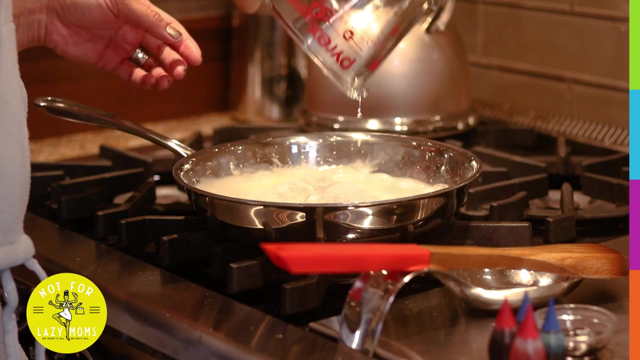 do is you'll pour in your oil. Next, I'm going to add my mixture- here The kids whipped up for us- of flour, Cream of tartar and salt. Finally, I'm going to add in my water Before the pan gets too warm. I. 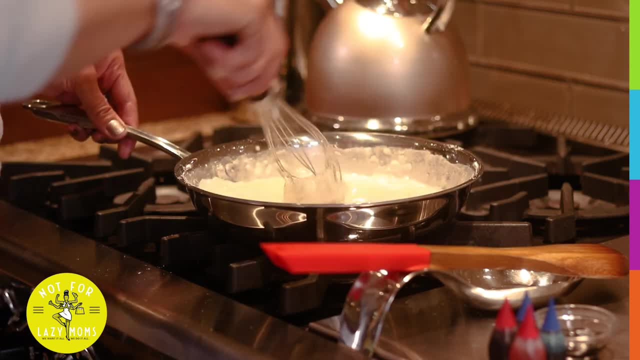 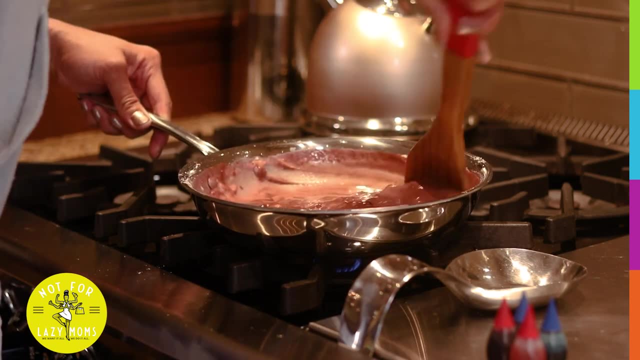 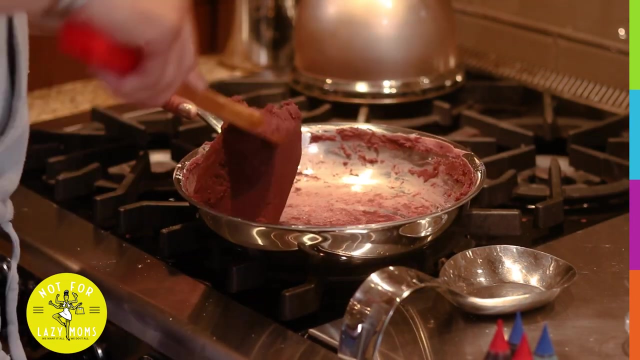 would just use my whisk just so I can kind of mix up everything, Add in the color, Just keep stirring, and keep stirring, and keep stirring and eventually a ball will form. You will have your Play-Doh. I'm going to let it cool off for a little bit and then I'll let the kids have some fun.